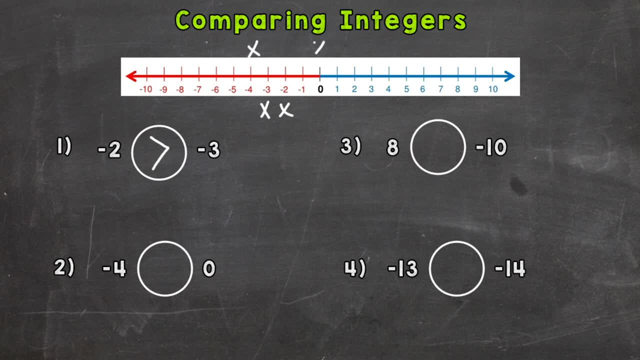 on the number line. I'll go above this time. So which is further to the right? Negative 4 or 0?? Well, 0 is, and that is the greater number. So we would read this from left to right: Negative 4 is less than 0, and let's think temperature Which? 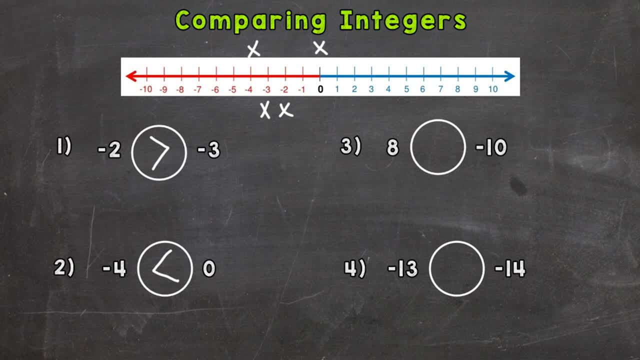 is warmer, negative four degrees or zero. Well, zero is Number three. a positive eight and a negative 10, which one's further to the right on a number line or think temperature. which is warmer, A positive eight is greater than negative 10.. 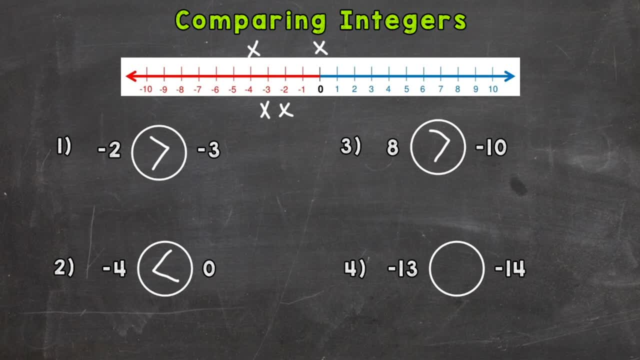 And then, lastly, number four: negative 13 compared to negative 14, which is further to the right on the number line? Well, negative 13 would be. Or, if we think temperature, which is greater, Negative 13 degrees is greater than negative 14.. 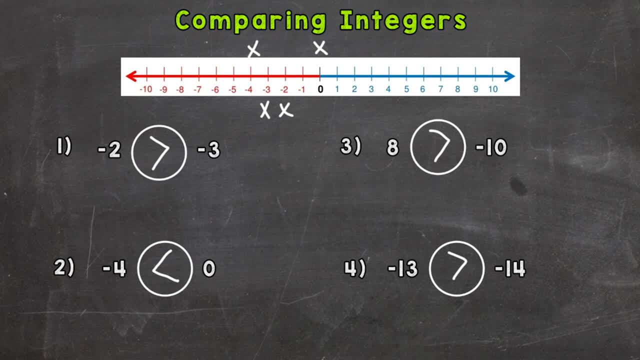 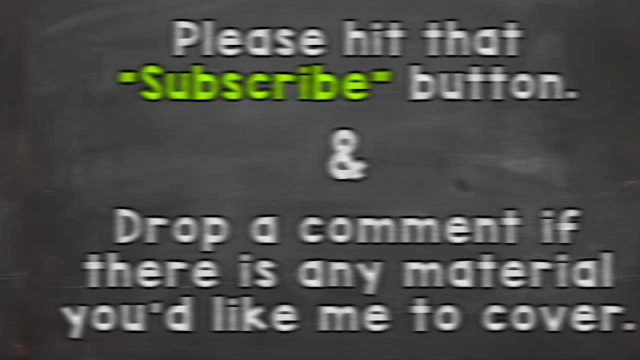 So there you have it. There's how you compare integers. Whichever number is further to the right on a number line, that number will hold greater value, okay, Or think temperature whenever negative numbers are involved. Thanks so much for watching. Until next time, peace. 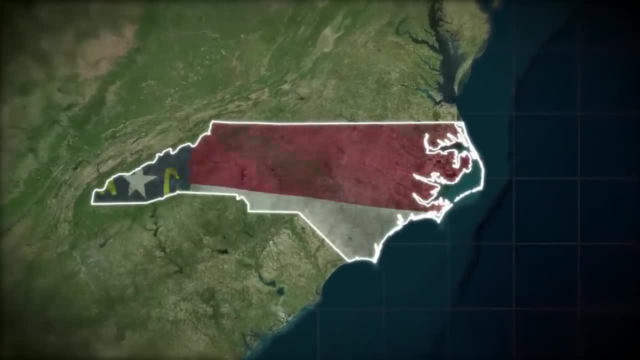 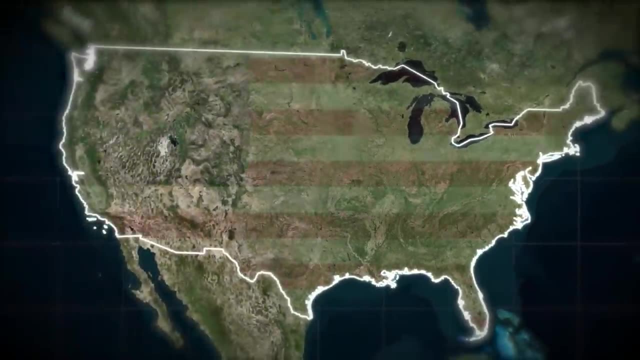 Did you know that the state of North Carolina saw an increase in population of 10% between 2010 and 2020?? For reference, the US population increased by only 7.4% in the same period. What's more? 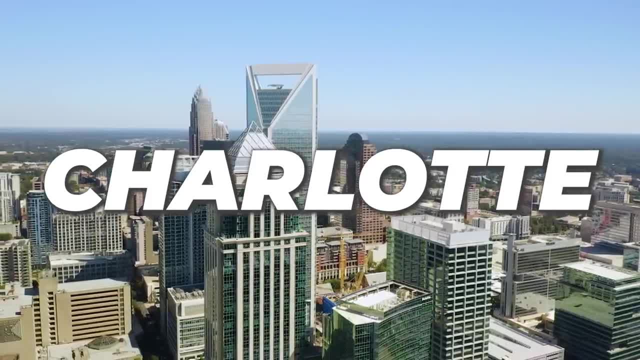 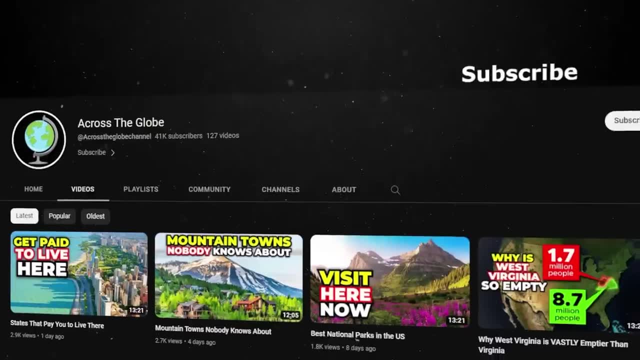 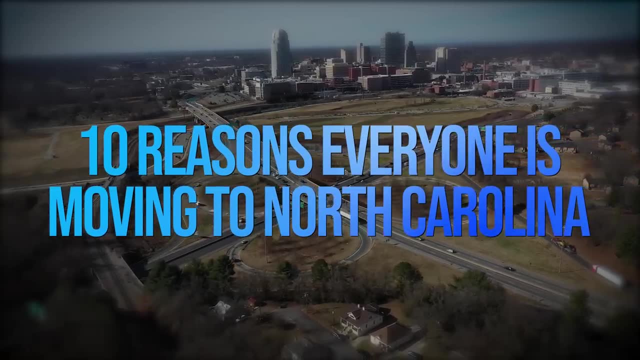 the cities of Raleigh and Charlotte are currently some of the fastest growing metro areas in the entire country. But what's the reason behind this growth? Well, today on Across the Globe, we're going to look at the 10 reasons everyone is moving to North Carolina. 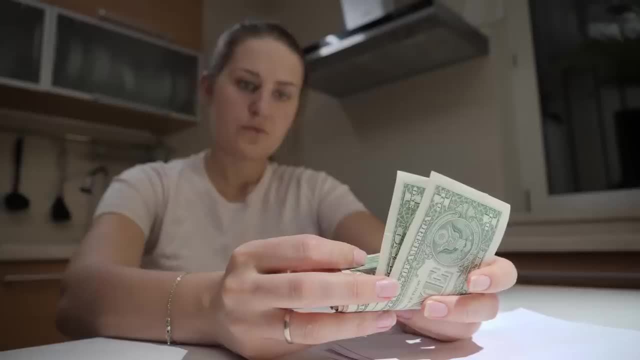 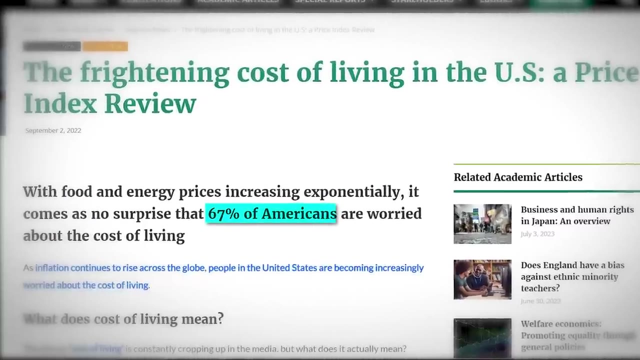 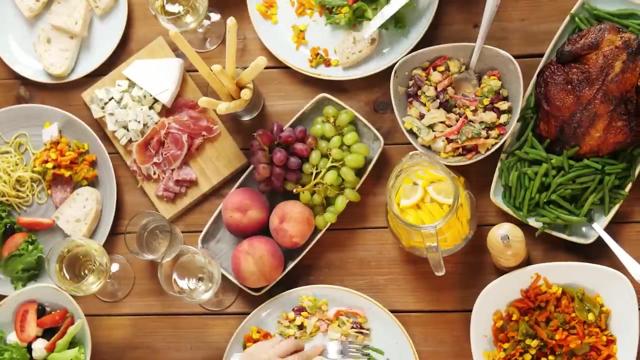 Number one: low cost of living. If you're like the average American, you've probably been stressed about the increasing cost of living. In fact, 67% of Americans report feeling concerned about this. The reasons for this are pretty clear: Food, for instance, has increased the most since 1979,.